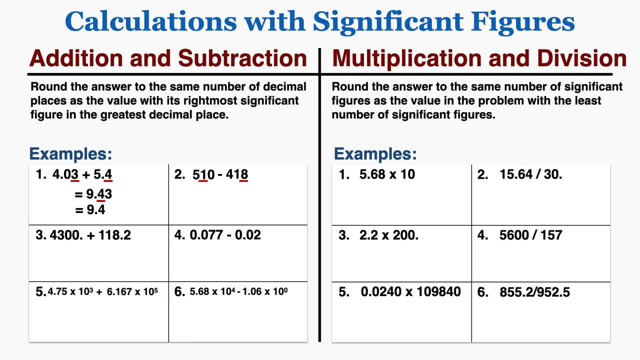 that's zero and 510 doesn't count as significant. So because that's bigger than the ones place where the eight is at, that will be the place where I round to when I do the subtraction. So I subtract and then I round to the tenths place, which gives me 90.. In problem three I do have a decimal point. 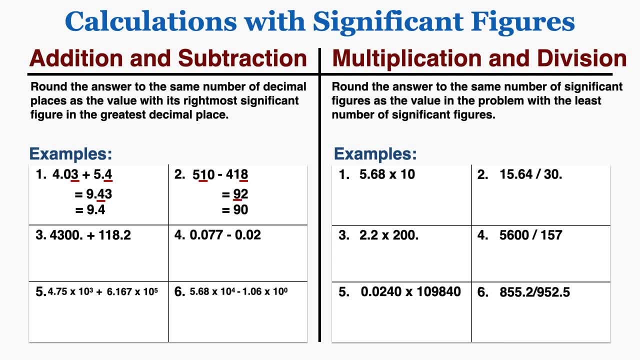 in both numbers. so those zeros in 4300 are significant. So I'm going to have to round to the ones place and then I round to the tenths place, which gives me 90. In my answer, which gets me 4418.. In problem four the first number goes down to the thousandths. 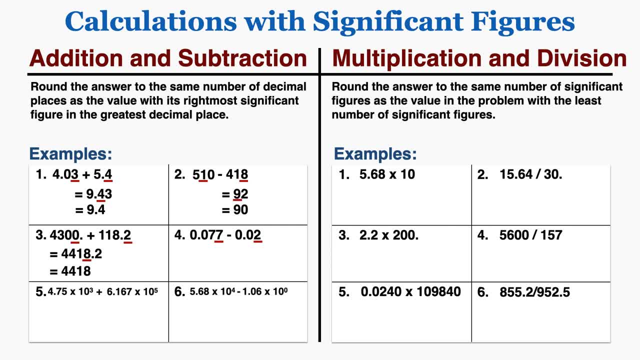 place and the second number goes down to the hundredths place. so I need to round to the hundredths place. So I need to round to this, which gets me 0.06.. Problem five is written in scientific notation, so I'm just going to rewrite that, just so I can see a little bit more clearly. 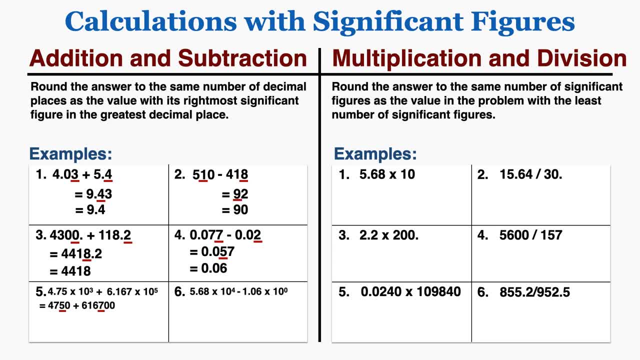 which decimal place each number goes to. I can see that the left number goes to the tens place and the right number goes to the hundredths place, so I'll round to the hundredths place. Problem six is also in scientific notation, and if I want to rewrite that in scientific notation, 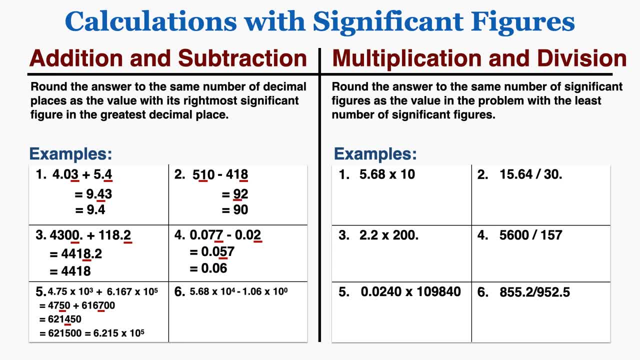 this is how it would look In problem six. I'm subtracting two numbers in scientific notation and I'll rewrite them so it's a little more clear. so I can see that first number is in the hundredths spot and the second number is in the hundredths spot. so I'll round to the hundredths spot. 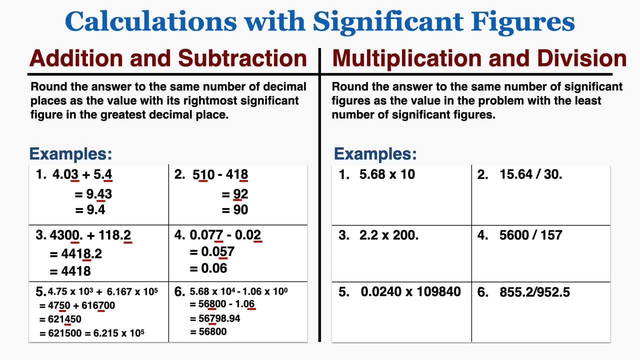 So that would be my answer. Moving on to multiplication and division, the rule works a little differently. When you're multiplying or dividing two numbers with significant figures, you're asked to round the answer to the same number of significant figures as the value in the problem with the least number of significant figures, so I no longer care about the decimal. 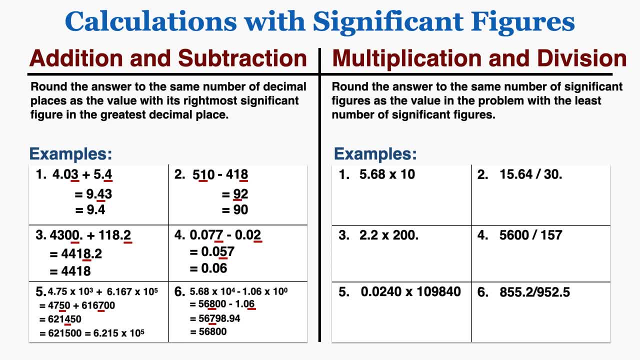 place. I only care about the number of significant figures and I'll always round to the least number. In problem number one, the first number has three sig figs and the second number only has one, so I need to round my answer to only. 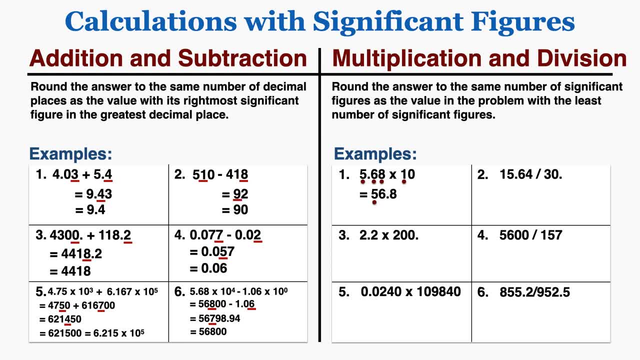 have one significant figure because that's the lower number of sig figs. So when I round that that comes out to be 60.. Problem two is division and I have four sig figs in my numerator and because that decimal point is there in the 30, I have two sig figs in my denominator. 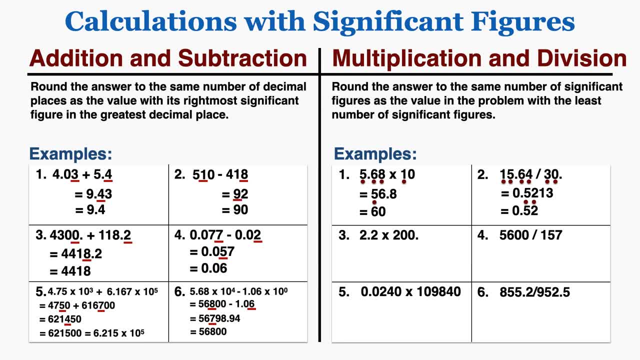 so I have to round the answer to two significant figures. so that would be the answer In problem three. I have a number with two sig figs and a problem with three sig figs because, again, that decimal point is there. so that means I have to round this number to two significant figures. 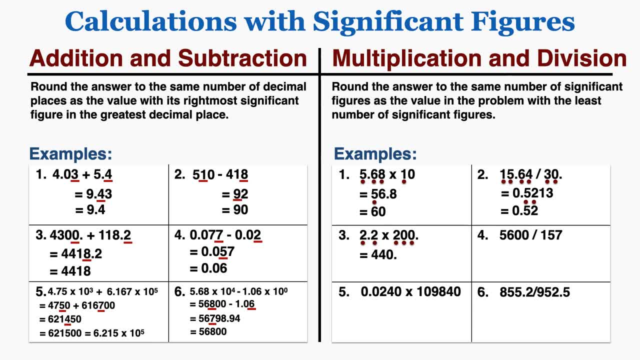 So this could be 4 4 0 with a decimal point after, but the problem is that that decimal point is making that zero significant. so I actually have to remove that decimal point so that the zero is no longer significant and I only have two significant figures In problem number four. 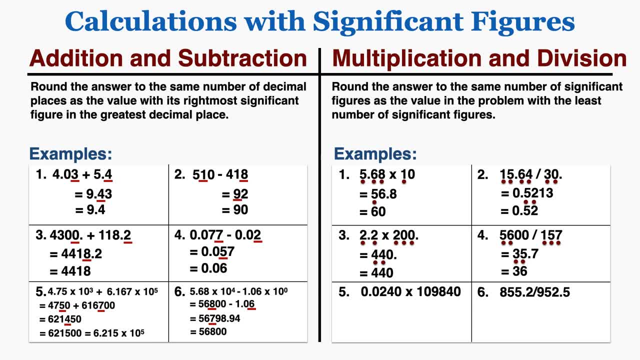 I have two sig figs over three sig figs, so I'll round to two. In problem number five, I have three sig figs times five sig figs, so I'll round to three significant figures. Finally, in problem six we're doing a division where we have four significant figures over four significant. 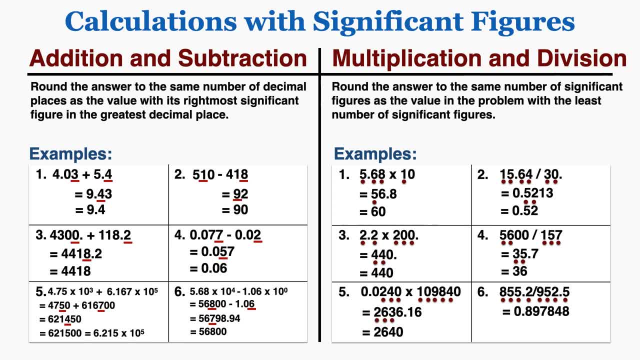 figures. so my answer will also have four significant figures. So this will be my answer. Rounding that to four sig figs gets me 0.8978.. So that's how you do multiplication and division while respecting significant figures. Finally, we can go on to powers and roots, The 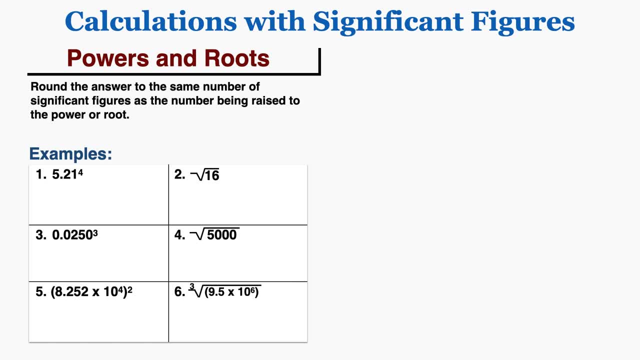 rule here is to round the answer to the same number of significant figures as the number being raised to the power or root. So we'll go through the examples. In example one I have a number with three significant figures being raised to the fourth, so I raise it to the fourth: power and. 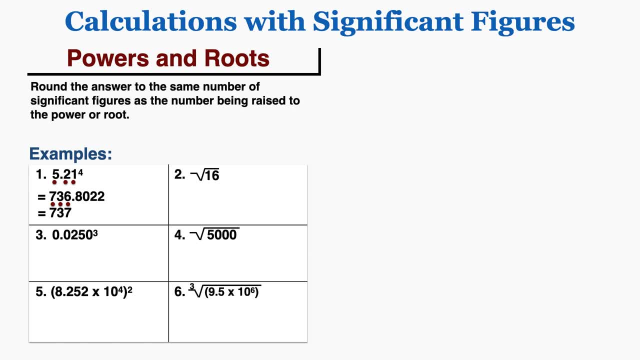 then round it to three significant figures and this is what I get. In problem number two, I have a number with two significant figures and we're taking the square root. So I know that the square root of 16 is four, but my answer has to have two significant 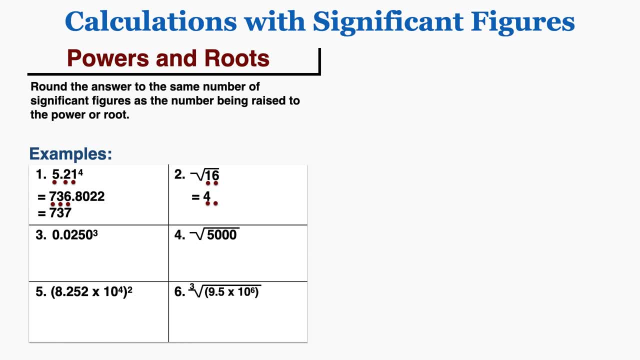 figures in it. So to add more significant figures, I'm going to rewrite this number as 4.0.. That would be the correct way of writing it so that it still has the same number of significant figures as the original number In problem three. this problem has three significant figures, so raising that to 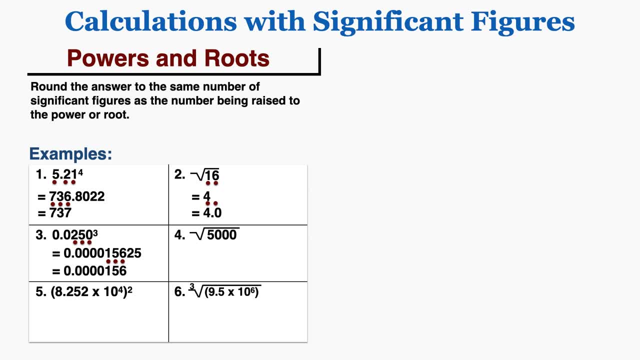 the third gets me this and I'll round it to three significant figures, and this is my answer In problem number four. this number only has one significant figure, so when I take the square root, I have to round this to just one significant figure as well. Number five: we